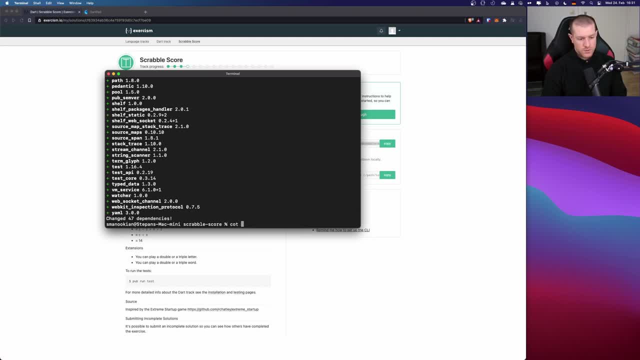 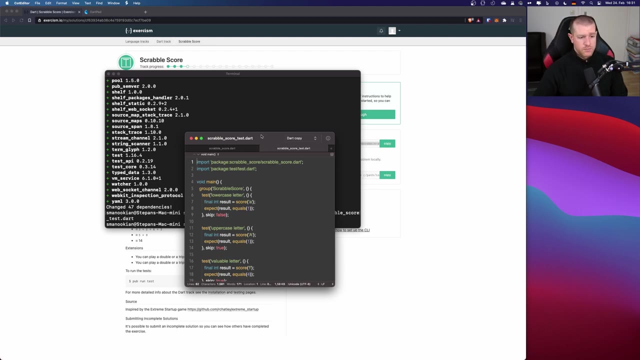 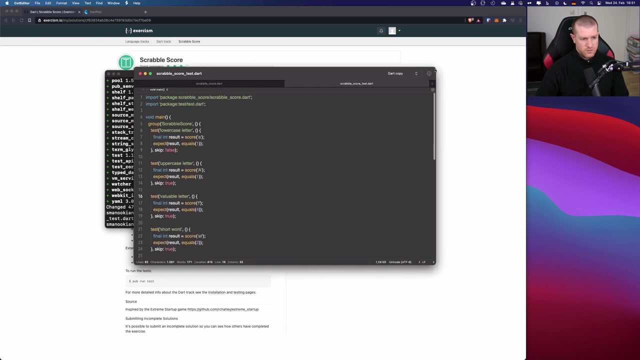 open the files and see what we need to do. I'll do it here, And you can go there via what is called a finder and then open the files on your own. But yeah, I'll do it like this. Okay, so let me do this bigger, Maybe. yeah, perfect. 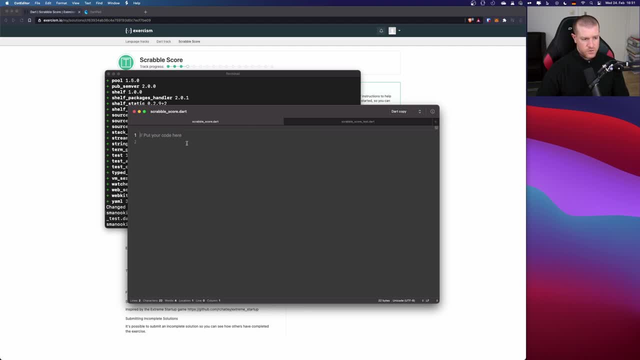 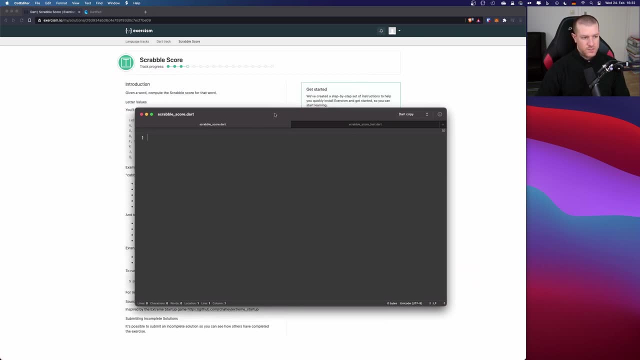 So this is our test file and this is our Scrabble score. So we have nothing in here and now. we need to see what the name of the method that we need to address and what are the, the return type and what is the parameter type, and so on. 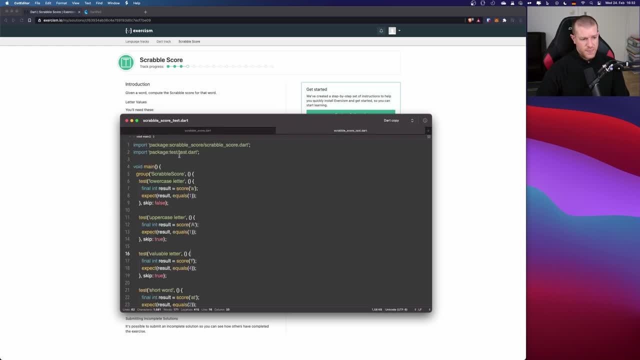 So we go to the Scrabble score test and then we see the different tests, like here's test one, test two, test three and so on, And in our test one we see there's a variable, It's an integer variable. It's called a result. 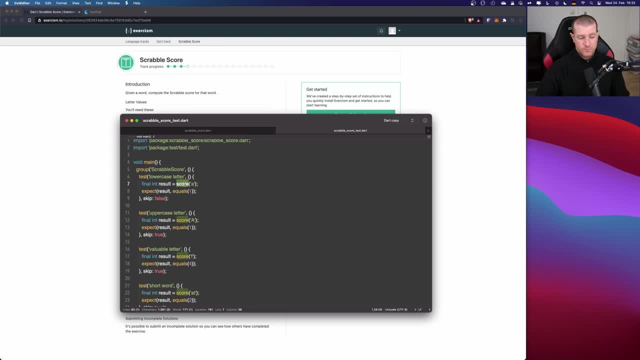 And you have a method here. it's called score. Okay, so our method should be named score, and it has a return type of integer and a parameter which is a string. Cool, Let's do all of that First. I'll copy a score here: 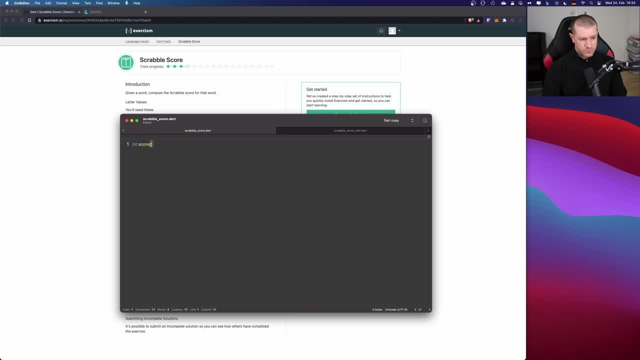 So we have an int score and string word. We say word, So let's do this, Okay, perfect. So what we need to do now is to think about how to do all of that. So if we go back here, we see we need to put 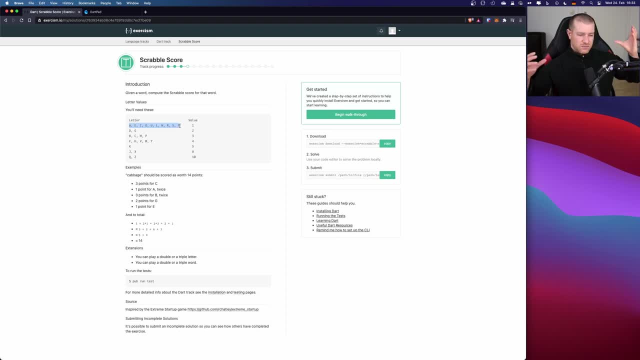 all of these in some kind of yeah, I'll, yeah, I'll call it a map. So we need to to map all of this. So we need to map the letter a to the value one and to map d to two and so on. So how we do that in Dart, We use map. 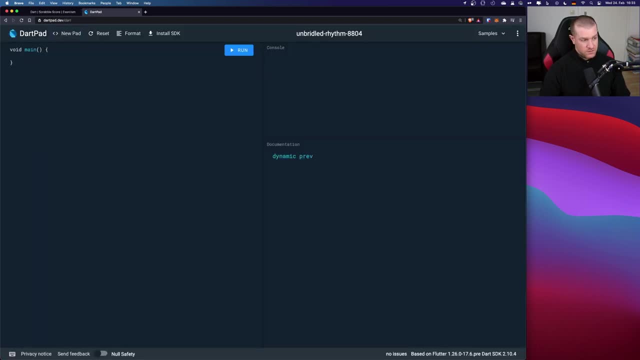 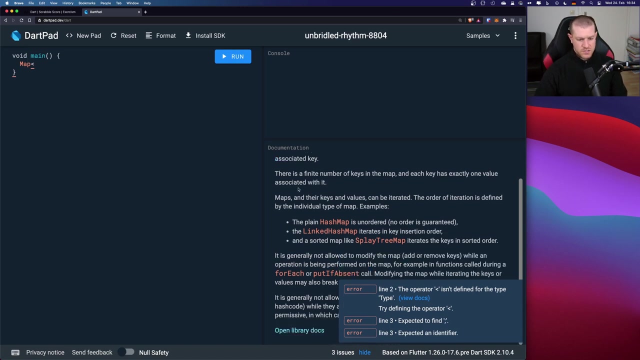 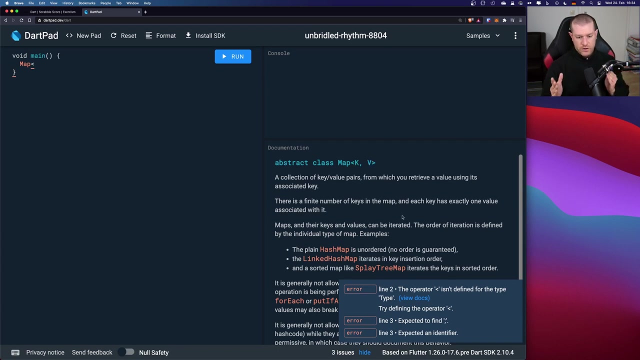 Let me go here and delete this and maybe make this bigger. Okay, so we use a map and we'll see what map does. So if I go here, so it shows me some information on this side And you see, here is k and v. So map is basically a key value pair. 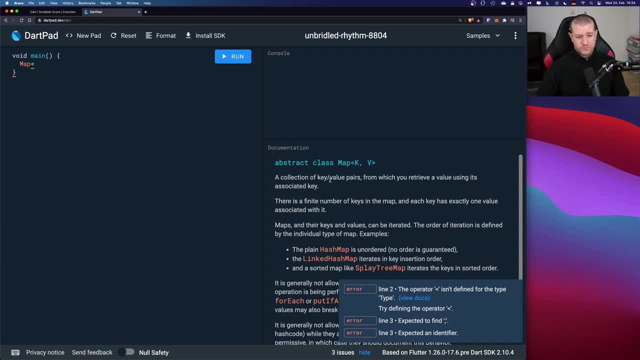 So it has a key value pair, So it's a collection of key value pairs. So it's perfect. It's written here, From which you retrieve a value using its associated key, So you have a key, and if you say, show me the value of that key, it gives you a value back. 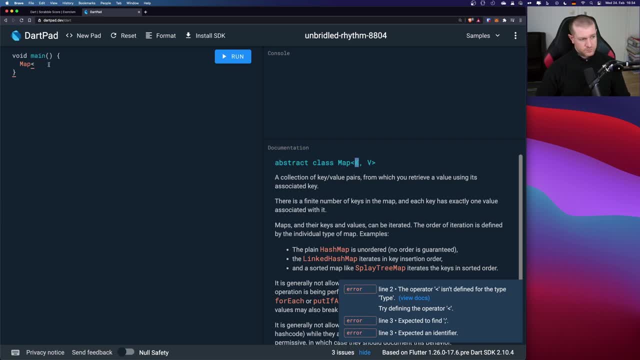 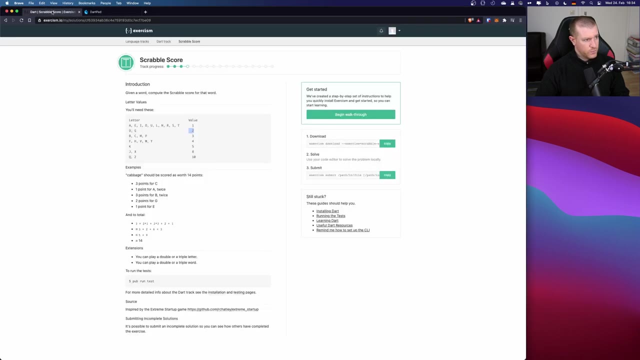 So, for example, I could have, or let's do the same example as we have. Let's say we have letters here, So if I go back to No, we go back here. So let's take: a is one okay and b is three and c is also three. 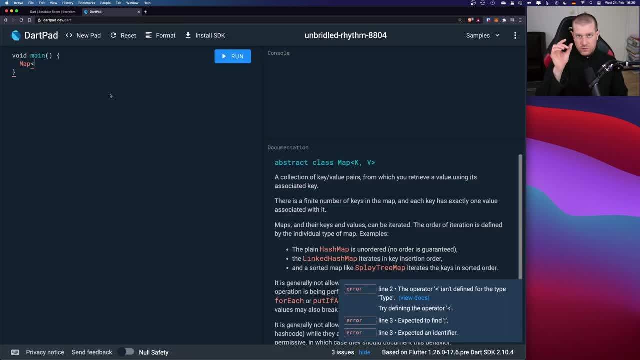 So let's do these okay. So what are we saying? We're saying a, b, c have value of some kind of integer, okay. So we say string Is our key. So the first one is a key in the map Comma. and now the type of the value: it is an integer. 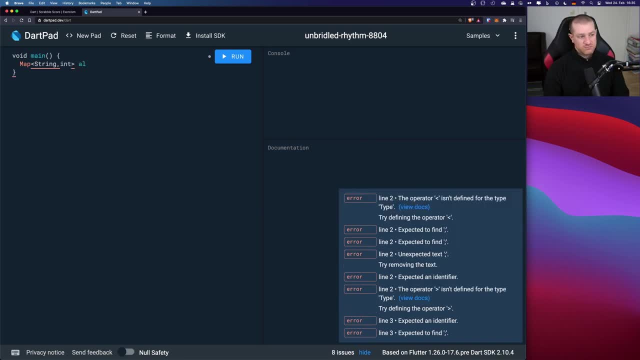 So, and we say alphabet to this one. so Okay, and how can we address this Or how can you Initialize this? basically, by putting everything in this squiggly brackets, And then we say: the first one is the string, our key, So we put a and then colon- I think it's called- and the value. 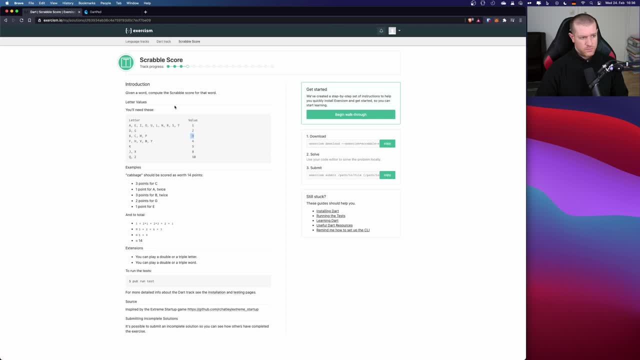 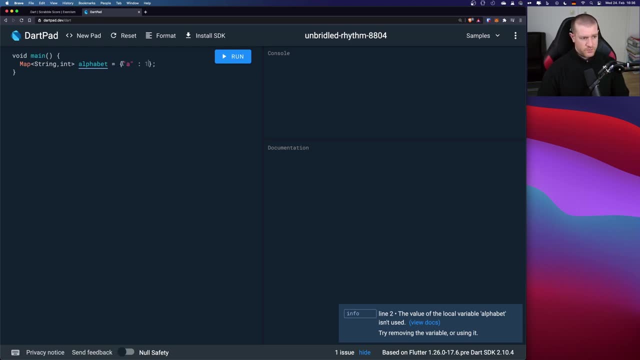 So we have: a is one, yeah, and the other ones are three. okay, So this is our first map key, Well, the first element of a map, And then we say comma if we want to put more elements in there, And then we go: b is three. 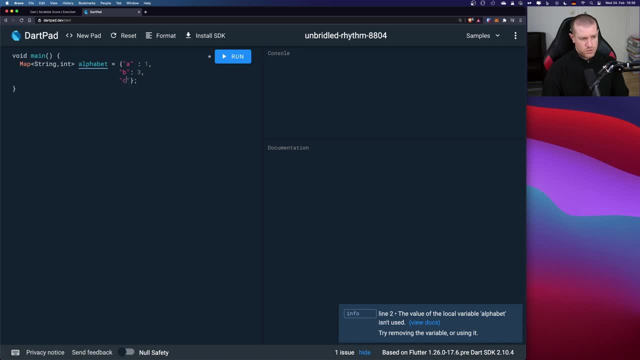 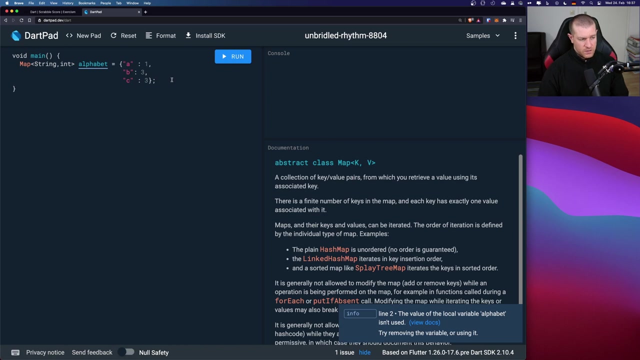 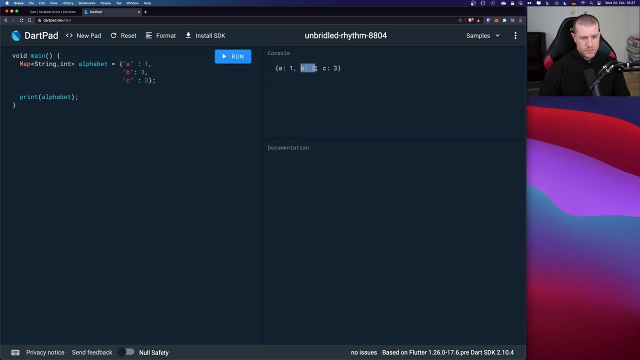 And c is three as well. So this is basically how you define and initialize a map. So easy like that. If I print, if I print that we'll see that we get a is one, b is three, c is three- cool, So how can I get each element? 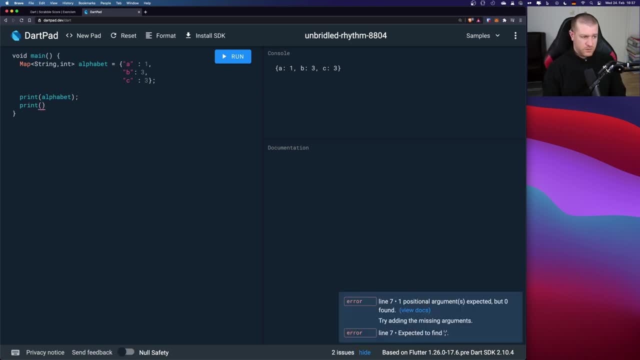 It's also easy, So let let print that out. So we say, yeah, I'll put a so we can see you. yeah, what are what are the results? are giving us back. So we have a and I will use the dollar sign here, and then this squiggly brackets: 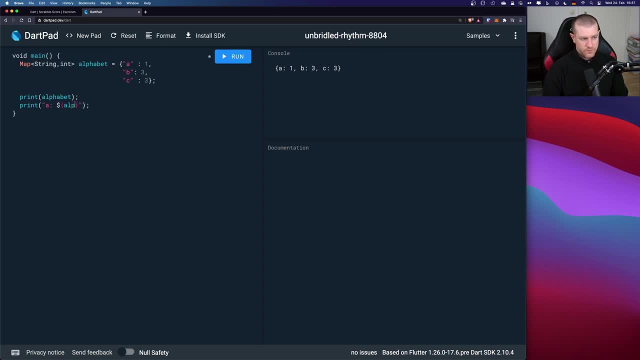 And then in there I'll say alphabet, And then now the these brackets And you have to put the key in there. So our key is a string and we say our first key should be a. Okay, so if I run this, I'll get back one. 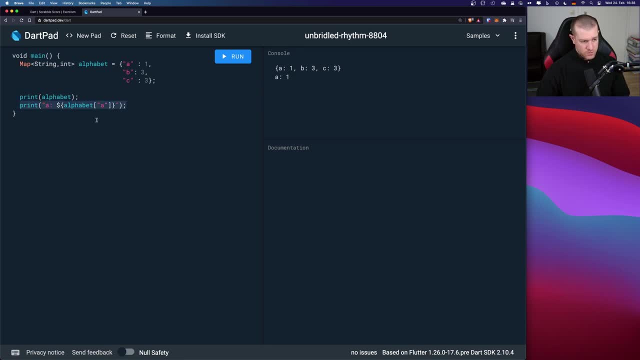 So, and if we do it to all of these three and we say our b And c, Okay, so it should be a one, b, three, c, three, Okay, so you just call your map, your variable, and then you put in and you put brackets in front of 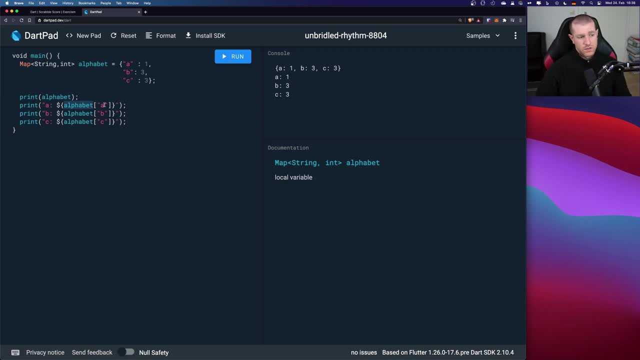 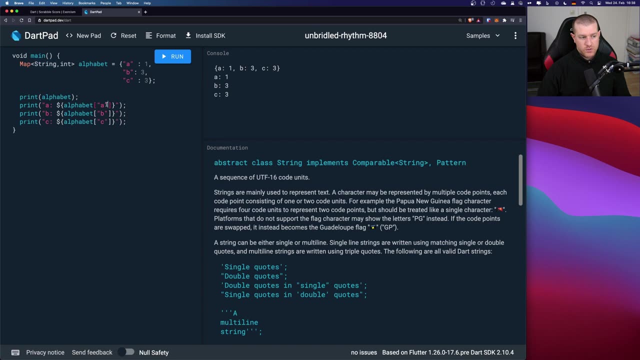 that and give it the key. So if you have, your key is an integer, for example, You put an integer in here, so maybe five or something like that. But we said our key is a string, so you have to put a string in here. 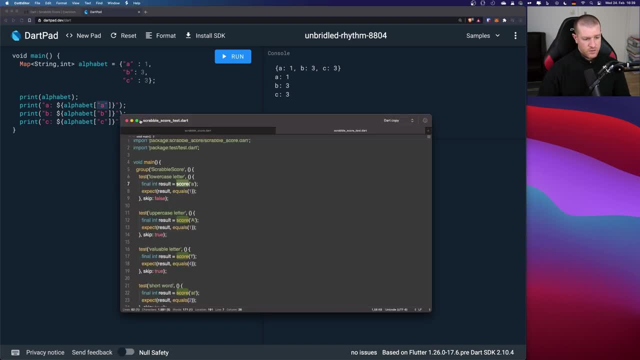 Cool. so basically we can go back here and, yeah, do our own map. I did that already, so I just need to copy and paste and you need to do it By your own. I'm sorry for that. so I put all of the alphabet, As they mentioned here, all of these letters, and gave them the values that they need. 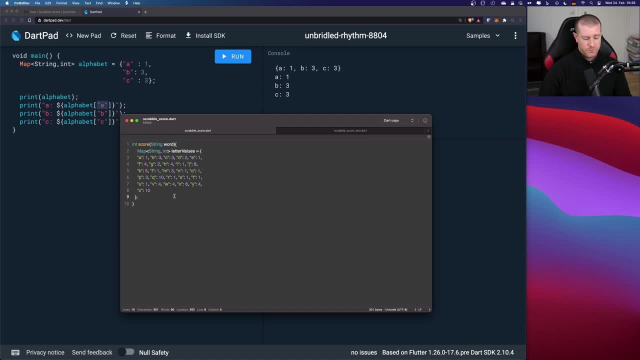 So okay, so that's our first step. So our next step is to go through them and then to add all the values together. So of course we can do, We can build a for loop or Or for each, or whatever, and then go through it and then at the end we say: 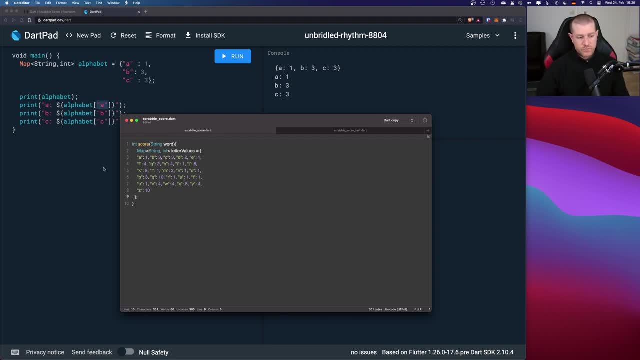 We add the values together and then, yeah, give that back. But as we progress in an exorcism, we need to learn new stuff. So, new methods, new concepts, new stuff, Yeah, so we will do it differently. We'll use something called fold method. 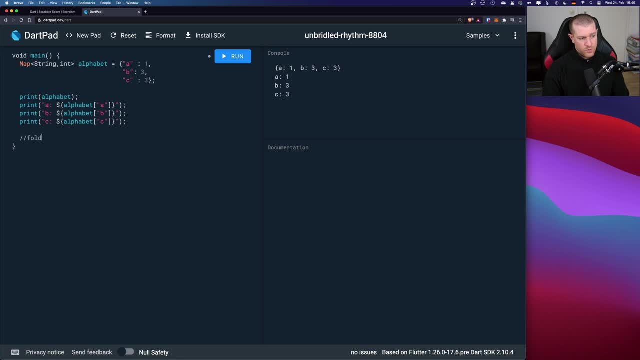 So we'll use the fold method. Okay. so what that is, we'll do a new example. Yeah, to address a fold. So, for example, I have a list of integer and I'll call this nums. So for numbers, and I give them, just yeah. 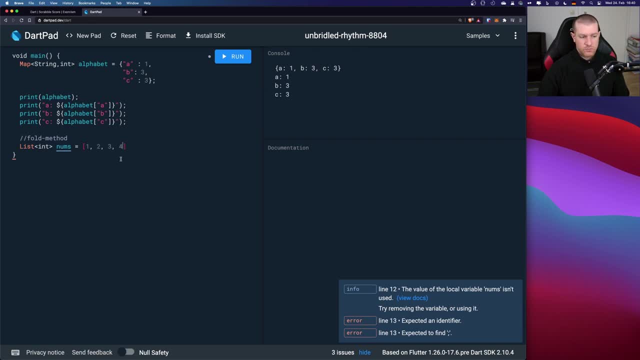 Yeah, these numbers, one to four, okay. So what I want to do is to add all of these together, So at the end we'll have one plus three, and one plus two is three. Three plus three is six. Six plus four is ten. 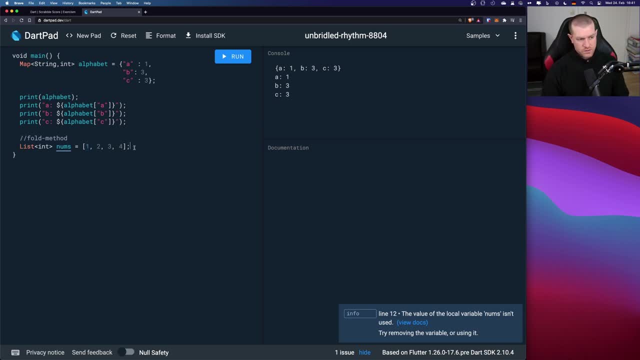 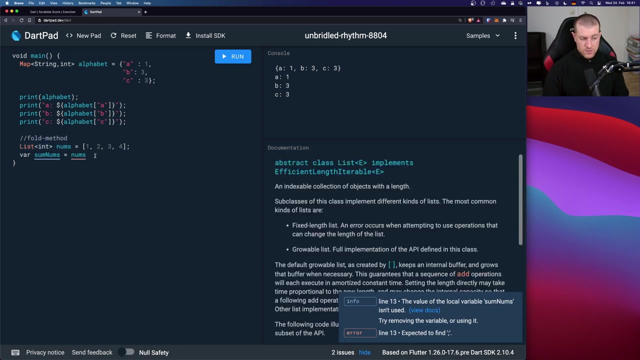 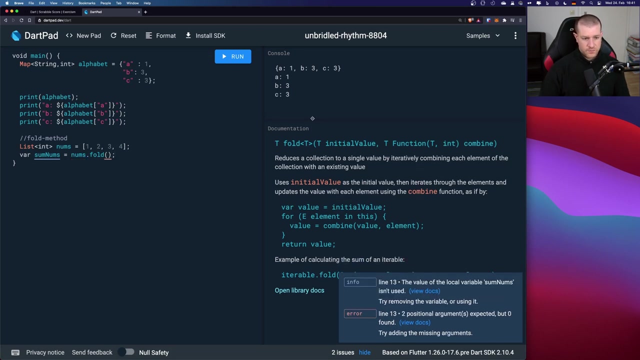 So we, it's the sum of all of these numbers. So we'll put this in a Some nums variable and then we say nums. So nums is our list here. Dot, fold. and now let us have a look what fold means. If you go here we say: fold reduces a collection to a single value by iteratively combining each. 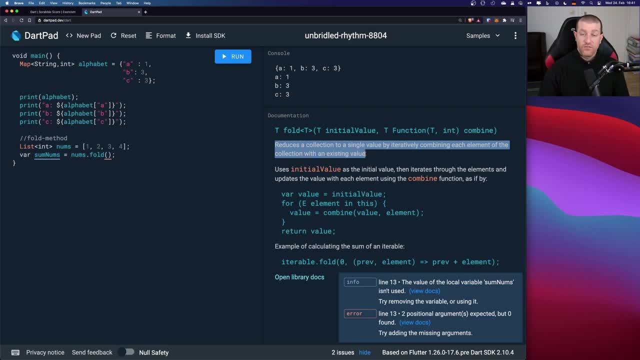 element of the collection With an existing value. So, and then uses initial value as an initial value, Then iterates through the elements and updates the value with each element using the combine function, as if by. and then here's the example. So, basically, this fold does exactly this with a form loop. 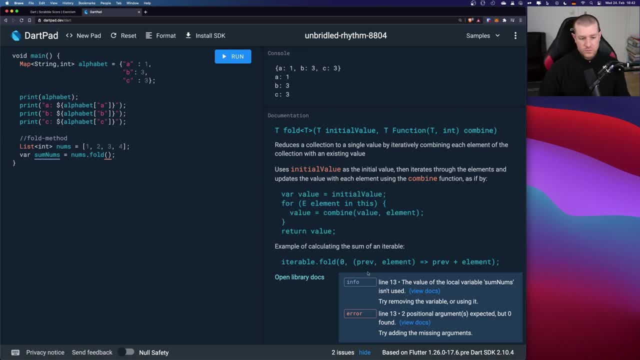 Okay, so let's go one by one. So we see here on the top Initial value. So here's an example And you see initial value of zero. So this is the value, and so it could be four, five, six, seven, ten, twenty one thousand. 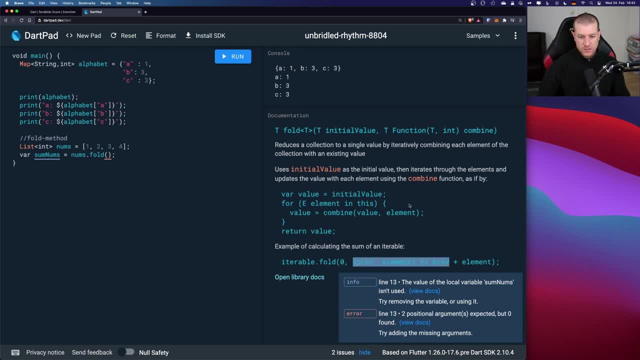 And then your function in here. So this function, Whatever it gives, like we say, we want to To, To, To To calculate all of these together. So we get ten back. So if you get ten back here, It added, adds this on top of that. 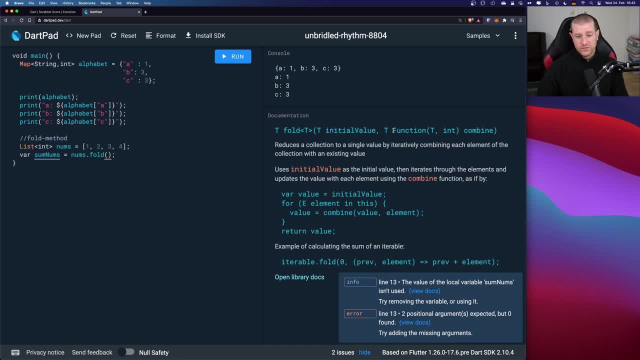 So if you have here initial value of four and you have ten here, it will be fourteen. So that's initial, the initial value, So the value from where you start. Okay, so it typically will be zero, So yeah, And then after that you have a function. 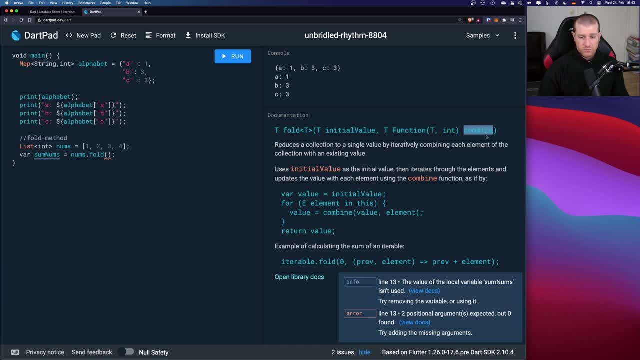 And then you have to combine them. Okay, so you have a function here. This, this will be our function, So we'll have preview And current element. So what is preview? Previous element. The previous element is The previous calculated element. 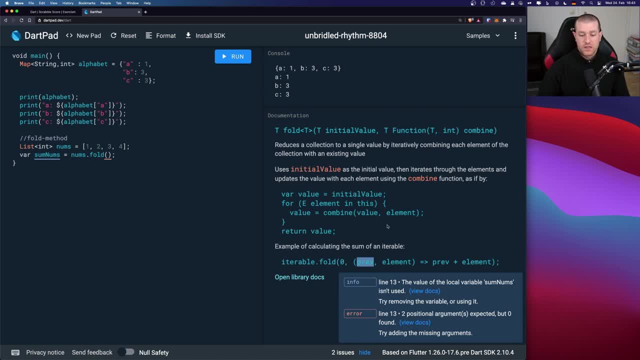 So what does that mean? The previous element here Is the calculated element over here, And the previous element here Is the calculated element over here. Okay, So the the value of previous value. it comes from the calculation of this Priv plus element. 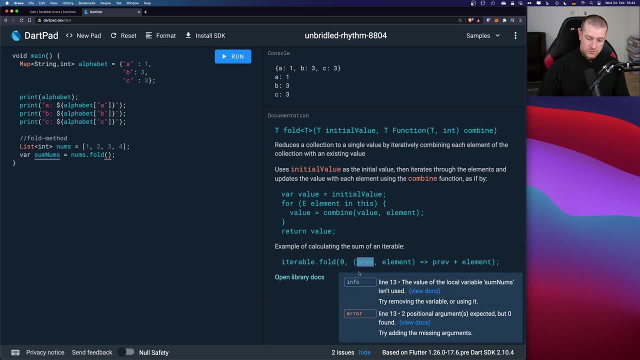 So whatever comes here out, it go here, and then you go With your iteration forward And the element is the, basically the current element of your list. No worries, we will do an example. Okay So, Okay, cool. So in here We say: 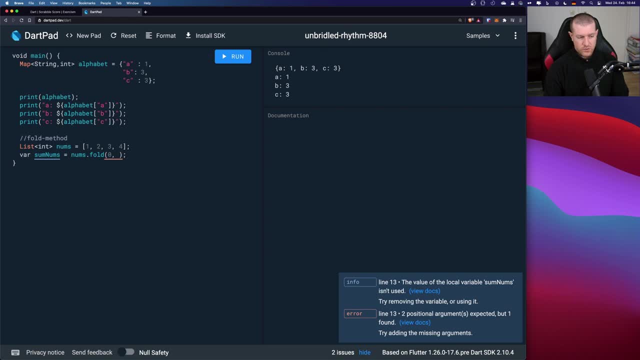 Our initial, Our initial value is zero. And then we said, If you go back here, We said we need previous and element, So I'll call it Priv. You should put it in a bracket: Priv And cur. So for previous element and current element. 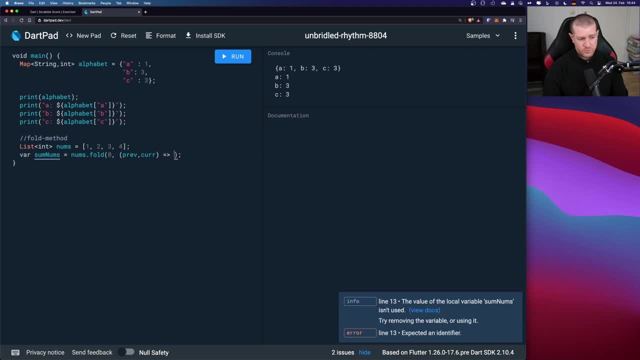 Okay, And then you Do an arrow And then you say Priv plus cur. So you do plus here because we said we need to add all of these together. If you need to multiply them, you can put multiply here. If you want to do something fancy. 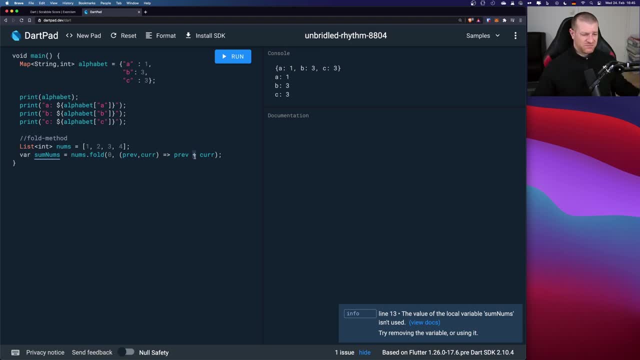 Like I don't know Some, some terrible math stuff. You can do it here And the, The Yeah, And then you get something out And then It goes back to priv And then You get a new stuff here. 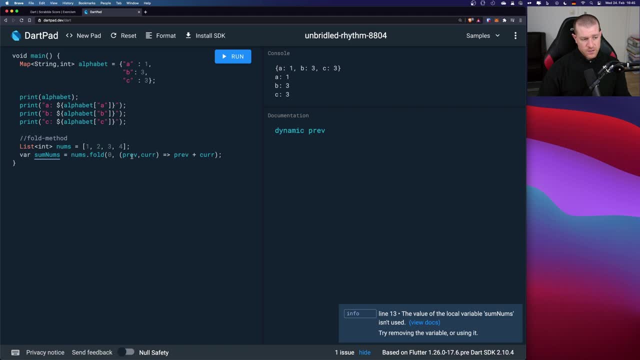 Okay, So Let's go one by one. So Now we have our num And At the beginning Our num Or our function here Is starting here. This is our current value, Which is here, And our previous value is zero. 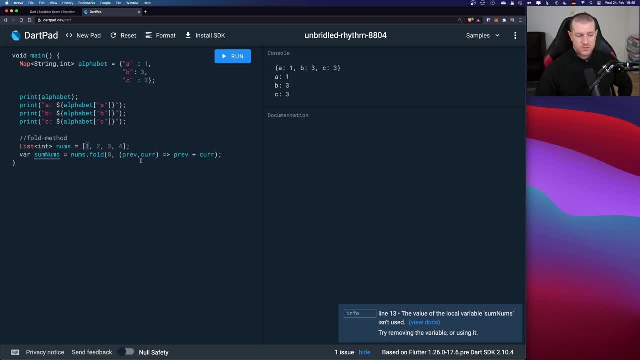 Why? Because we didn't calculate anything here. So initially it will be zero. So we will have Zero Plus One. It's one. So now we calculate this. Now the next iteration occurs. So we have: the current value is two. 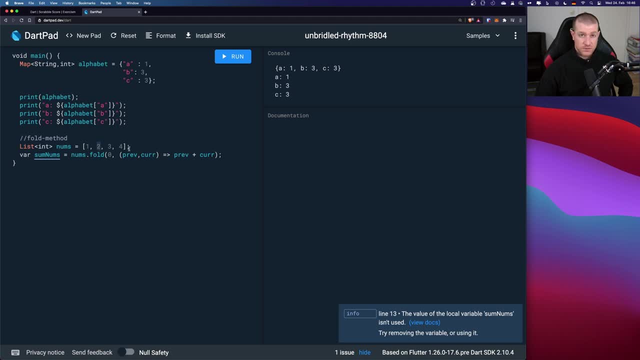 Here's two. What is our previous value? It's one, Because we calculated In the last iteration. We calculated Zero plus one as a previous, plus current Is one. We put it in here And the current is two. One plus two is three. 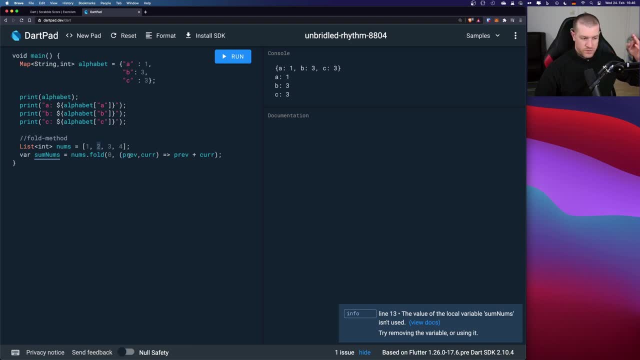 And now we get three here. We put it in previous in here, So we have three, Our current is three, And then you add it, You have six. You put six in here, Current is four And then you say four. 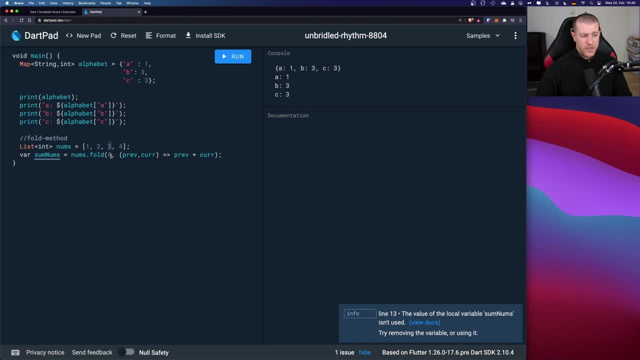 Six plus four is ten, And then you give it back If we have here something like Three, or, yeah, Forty three, And then you say you have ten here, So you add the ten to this, So you have fifty three at the end. 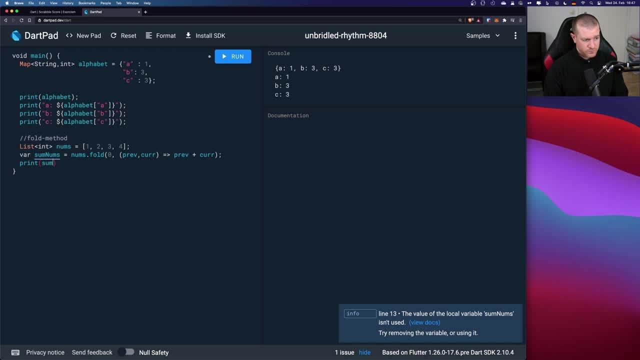 Okay, cool. So let's print this and see What we got. So Cool: We have ten Perfect. That's exactly what we said. So Let me, Oops, Come on. So Okay, so I'll. 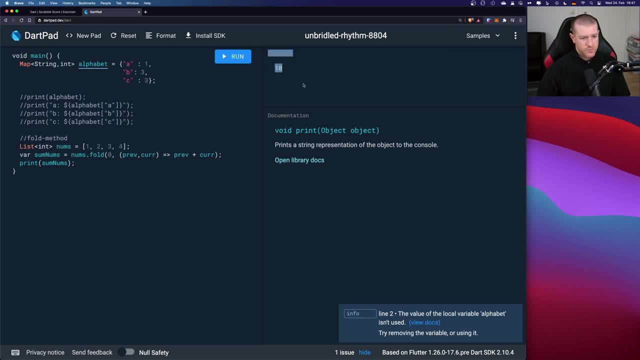 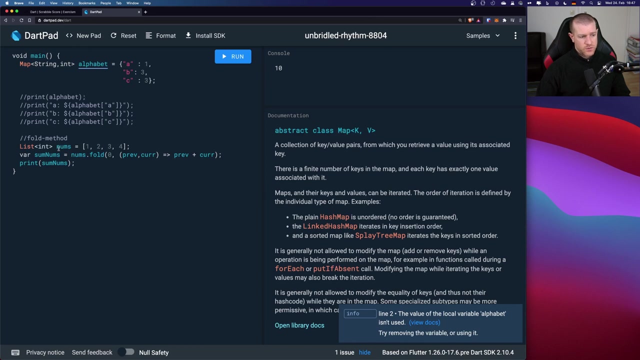 Yeah, Comment this out. So we have ten. Okay, cool, Perfect, So this is basically what we also need. So we need to have a map and we should go through the map and then add everything together. So basically, just fold. 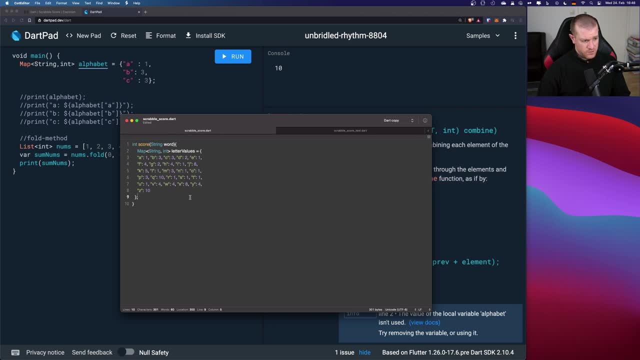 Okay, perfect. Well, my voice cracked there. All right, So we need to return something, So I'll comment everything up here. So let's say: you will get Steve, for example, as a word like this. Let's say like this: 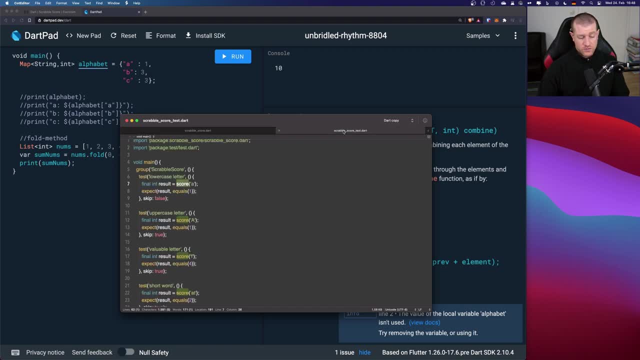 I know the capital letters because if I go back and see the second test is an A with a capital letter and it should give back one, And if you see here a, It should give also one. So there's no difference between capital and small letters. so that that's also important. 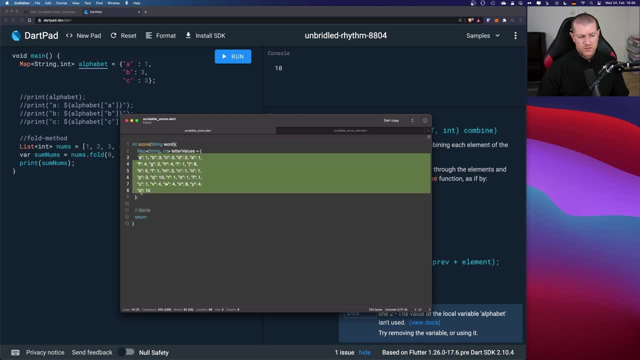 So how can we do that? Because we we are using only the small letters here, not the capital letters. So, and if you get something like this And it it takes, it takes the capital S and goes through your list and says: I don't know what that is. 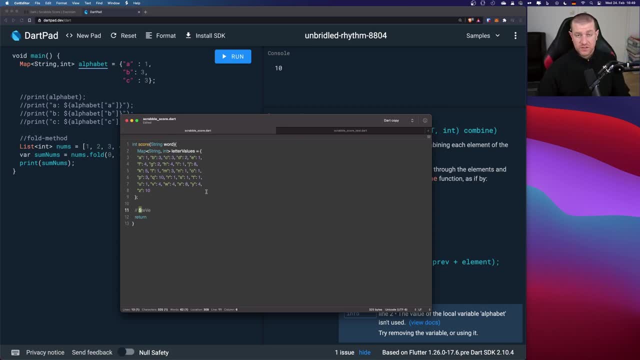 It's a capital letter, It's a capital S. It has a different value, but I don't know what that value is, And it gives you null and then you get error and everything explodes. So make sure that the first thing that you do is to take your word, the word that you get from here, your parameter, and say to lowercase. 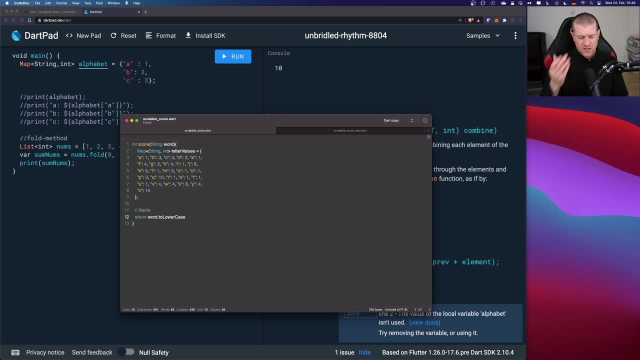 Okay, Or you can do it also in uppercase, if you convert all of these to uppercases And then you need to put everything in uppercase, but I'm using lowercase, Okay, so that's the first thing. you do: Everything in lowercase. 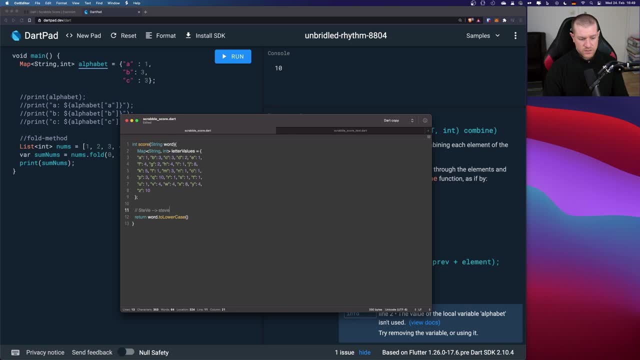 So what's happening now is you get something like this: Okay, next step is to make your word iterable, So you can iterate Through each letter of that word. So basically to make a list out of it, as we have here with our nums. 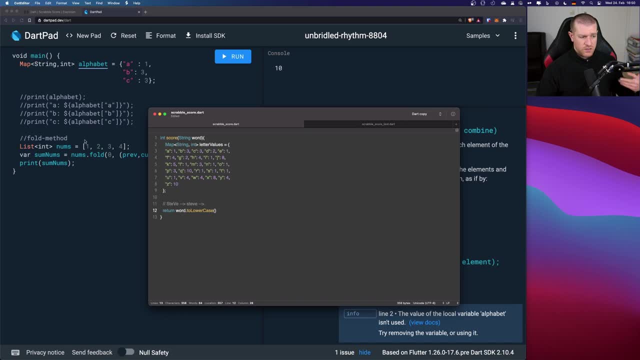 So with our variable nums, And it has numbers as a list, So we need a list. How can we do that? That's also easy. We say split And then in here we say, where should it split? So 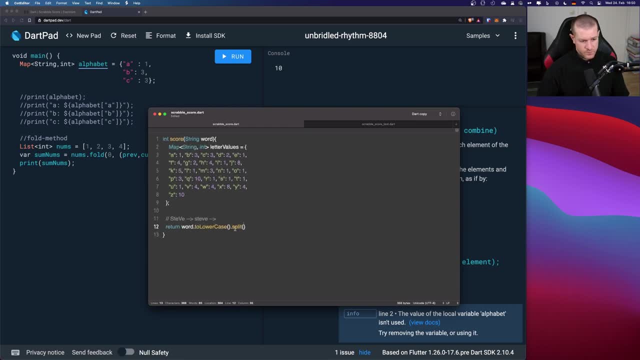 For example, if I have like Steve is the best and I need to split it every like I need to split these words, I will do something like this: I will say split and then give it the empty space. 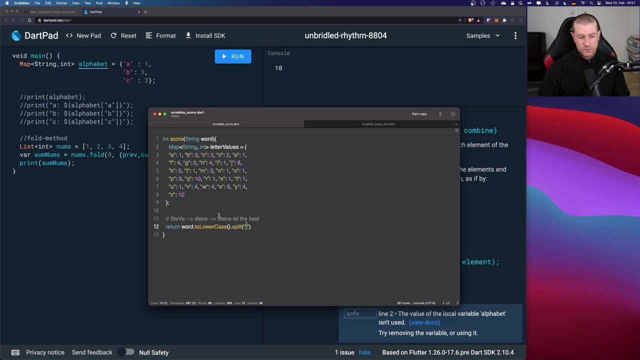 So Okay, Okay, Okay, Okay, Okay, Okay Okay, The split method will go through here and say, Steve, oh, there's an empty space. Split is what is, what is this? Is split, the split best. 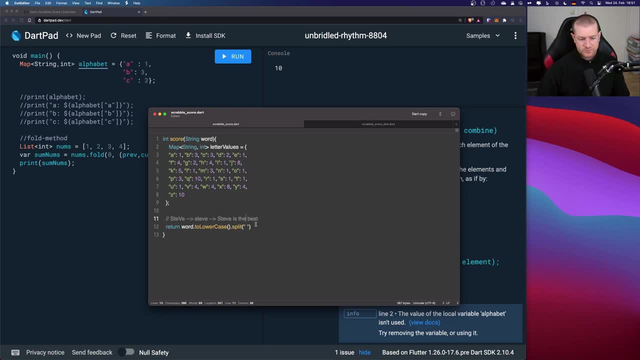 Okay, So it goes one by one. If you have a you want to like to split by comma, you say, okay, comma. So this is your first word or string, And then this: this: This is the second string. 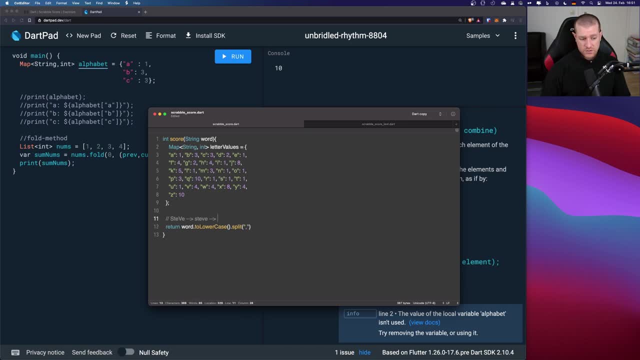 But we don't have that at all. So we have a word. So how can we split a word? We just give it an empty string And by doing that, So an empty string, not not like this, Really an empty, empty string. 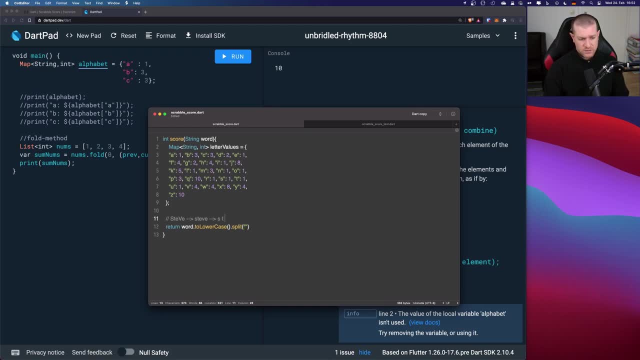 Okay, So now. Now we have something like this: S-T-E-V-E, So Okay, Okay, So Now it's our word split, And now we can iterate through each word, each character of this word. Okay, And we use that by using fold. 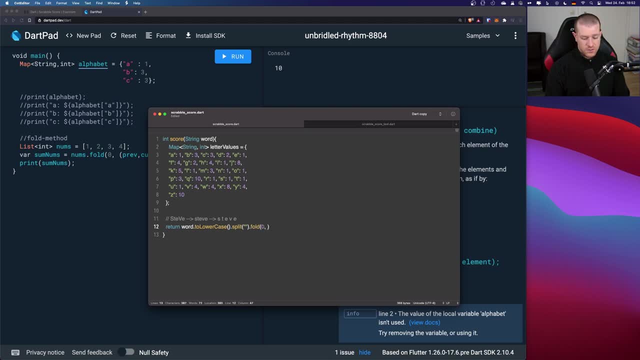 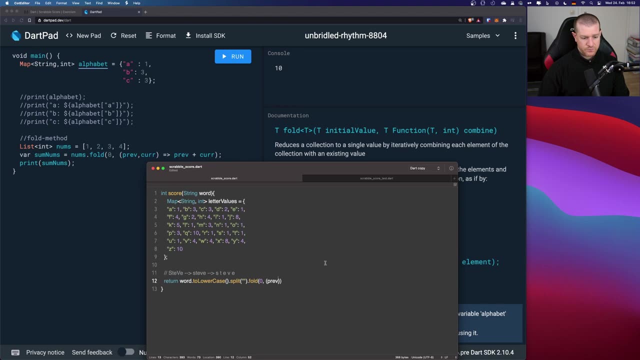 So we say: fold, Our initial value should be zero. And then we have our previews. Let me do it like this: Yep, Okay, So we have our preview, previous value and then our current current value, And we say previews. 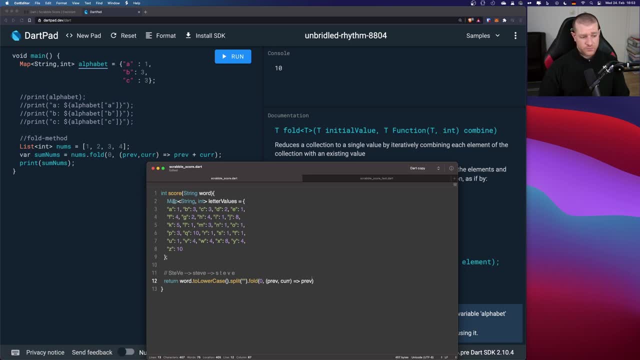 And now we should take the value of, of, of, of the letter values of this variable, So the map variable. So how can we do that? It's also easy: We say that letter value So this one, And we give it. 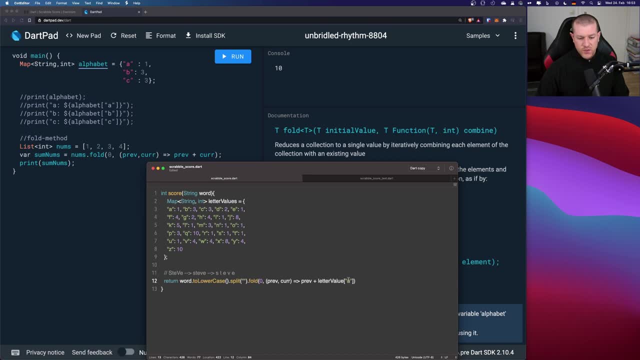 So, sorry Or yeah, If I put an A in here, it will take the the value here. So we have our curve. So this is our current value, This is our current key. So we put it in here and don't forget to semicolon. 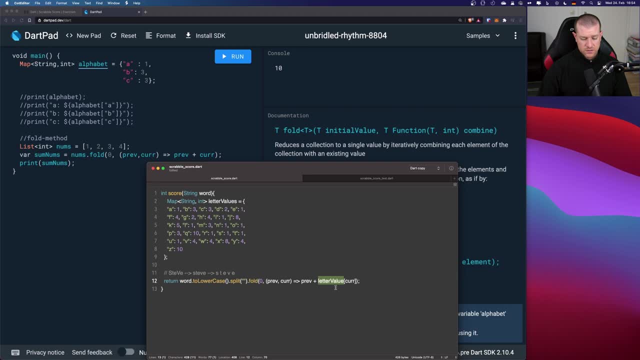 Okay, So basically the letter value is our map as you see here, And then the curve is our current um character, what we get here. So we get S and then it says letter value S And then it checks: here: S is one and it gives you one back. 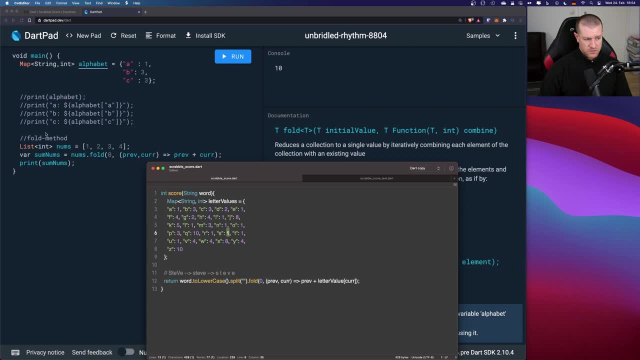 And then all the addition stuff, basically like: uh, here in our DART, DART pad, um shown here, Um, yeah, it gives you exactly that, what, what we need. Okay, cool, So this should work, hopefully. 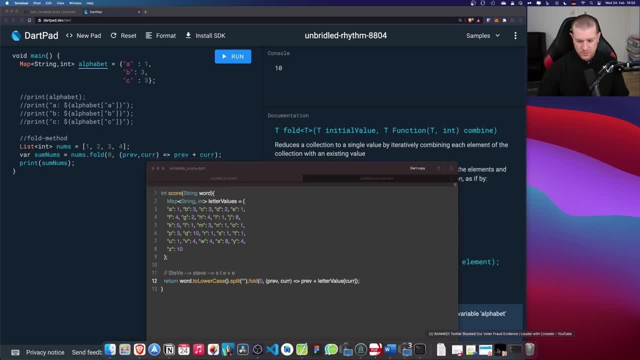 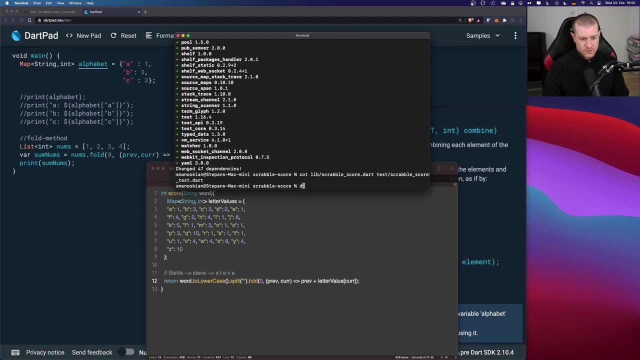 So we go back to our terminal: Uh here, Okay. And then we do the test and say DART, run test and let's see if everything is fine or we did some errors, but it should be, it should be fine. 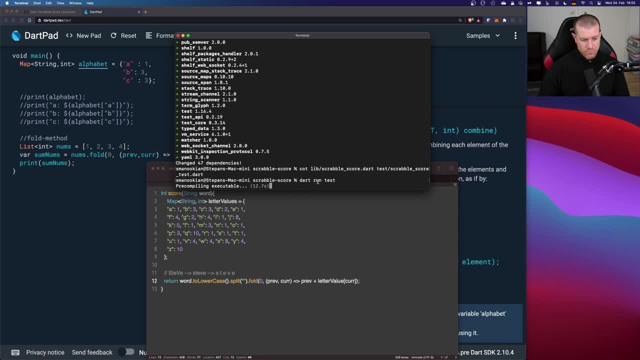 Let's see. So yeah, as always, there's always an error. Okay, So uh, yeah, there's. uh. I need to copy this, So I'm missing an S at the end here, but I will paste this all. 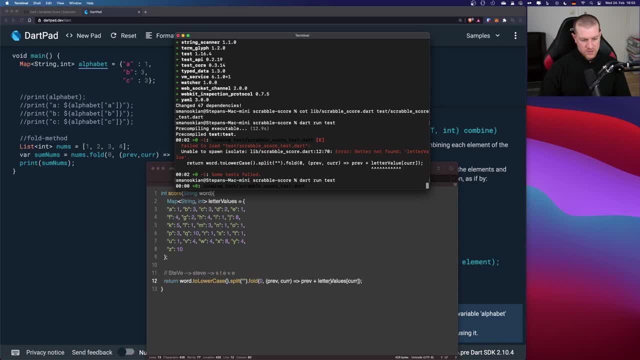 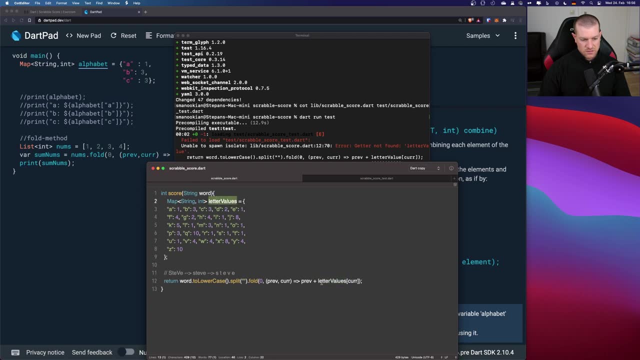 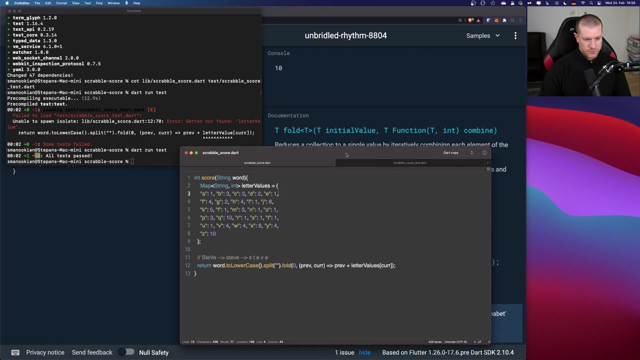 So let's do that again. So yeah, just yeah, just just see, uh, how these things are written and stuff like that. Okay, So we get plus one and 10 are skipped. Okay, perfect. So when I do this, if I go back to our test file and copy this false and then put it basically, 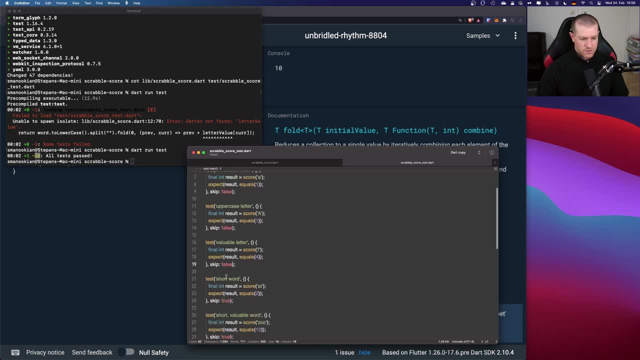 everywhere it says skip false. So it go through all the tests and hopefully at the end, Okay. So let's see. Okay. So let's see We get everywhere Correct. So it should say plus 11. Okay, Perfect. 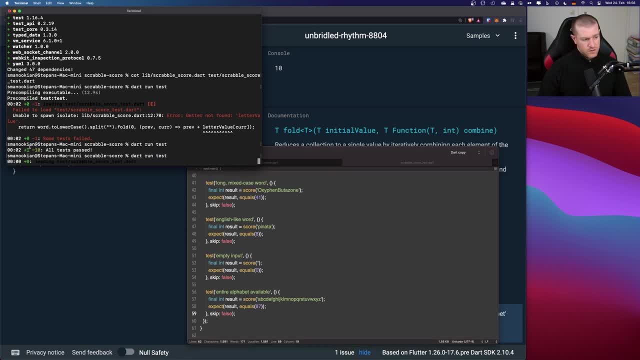 So that's it. That's Scrabble score. I hope you learned something new. So we we had a look at um map and then also uh uh fold, And these two are really, really useful. So let's see. 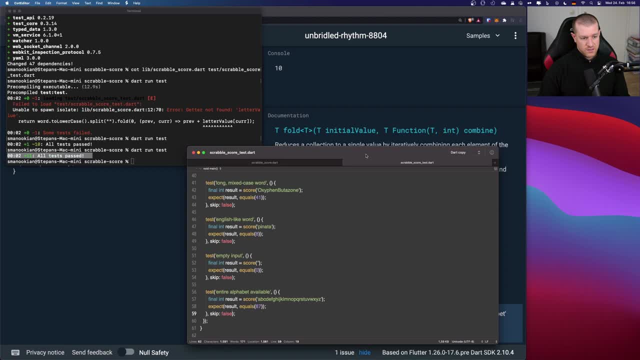 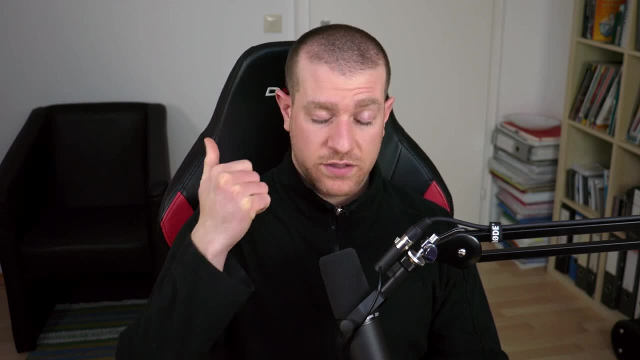 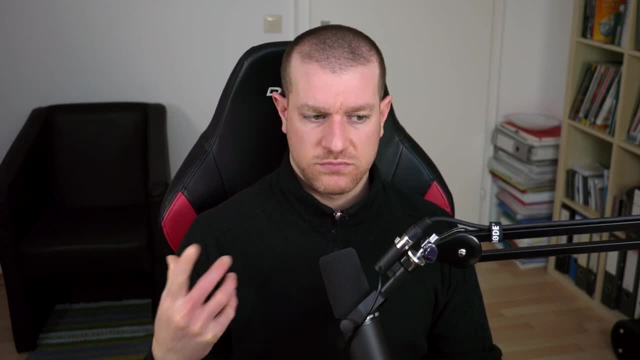 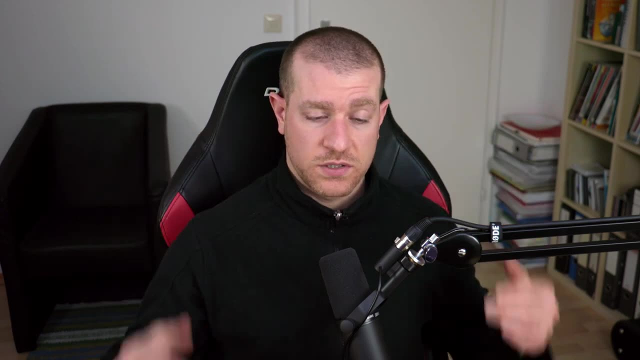 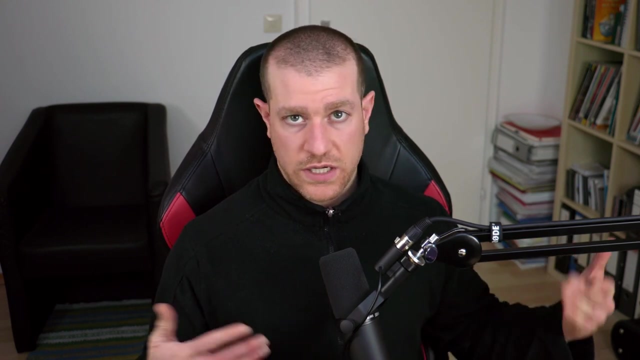 So let's see, Okay, So these two are really, yeah handy um stuff to have and to know about. In the future we will use something called map is basically the same as fold, but it can do also other stuff. 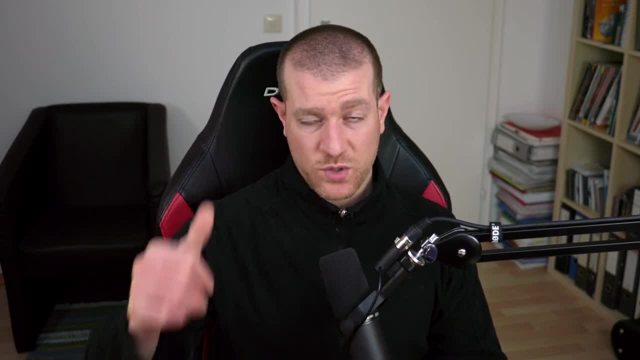 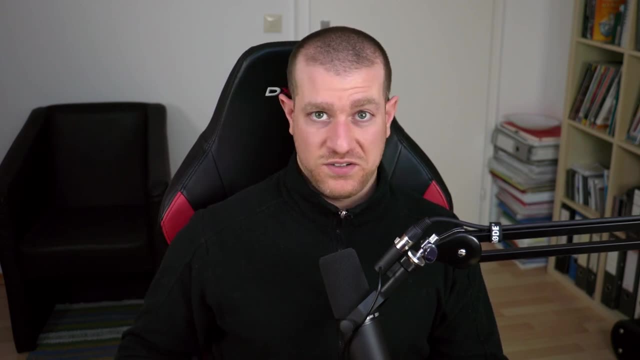 So, yeah, if you're learning something, show me with a like and subscribe to my channel. I will do other um exercises and hope to see you next time, Steve out, Ciao.